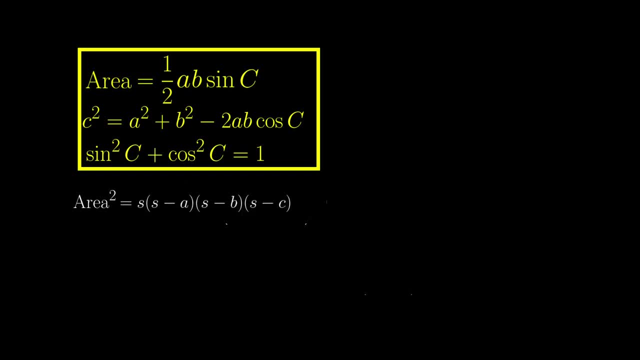 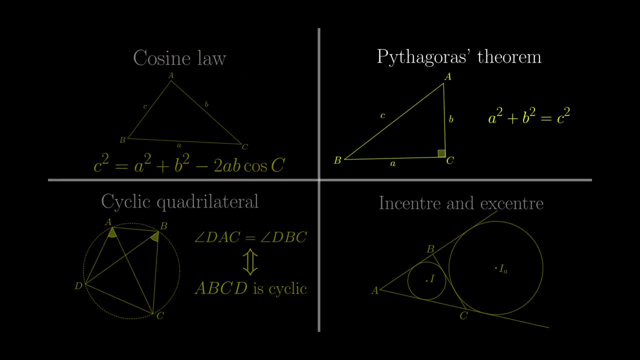 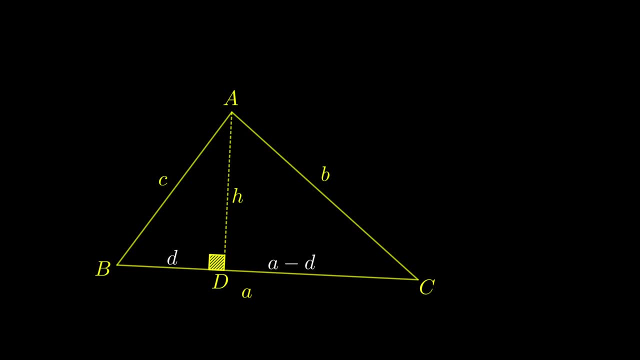 Consider this triangle where we split the segment of length a into two parts by the height, Based on Pythagoras' theorem, we have these two relations. Subtract the second equation from the first, we have this equation, which can be rearranged as follows: 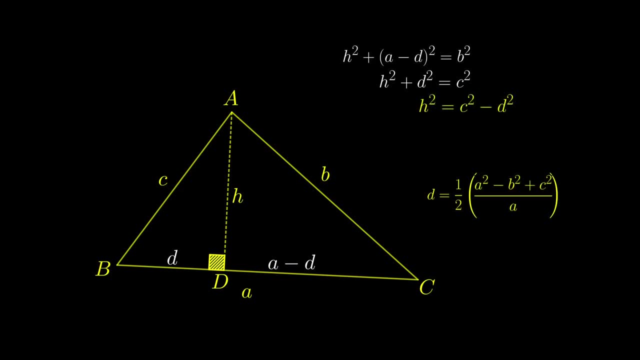 Subtract the second equation from the first, we have this equation, which can be rearranged as follows: Now the area is actually half a times h, So we get this formula and the algebra from now on. The formula from now on would be very similar to what we have done above, so I don't bore you with it. 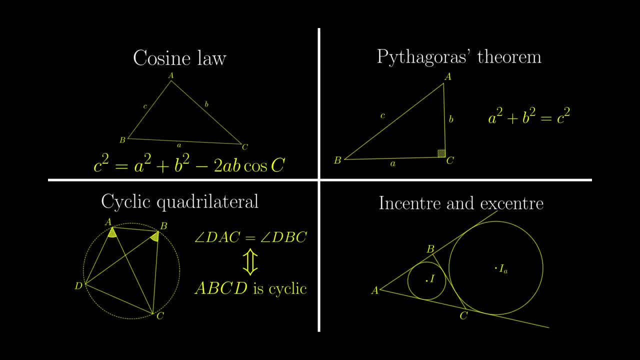 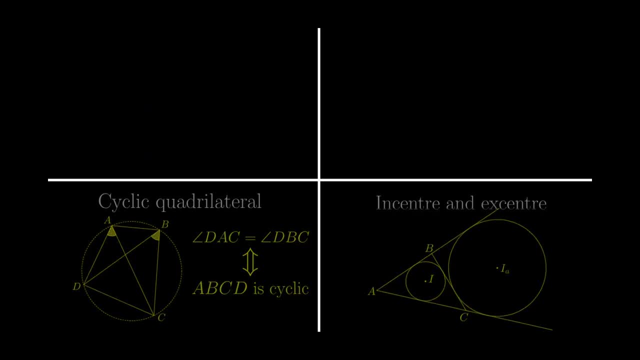 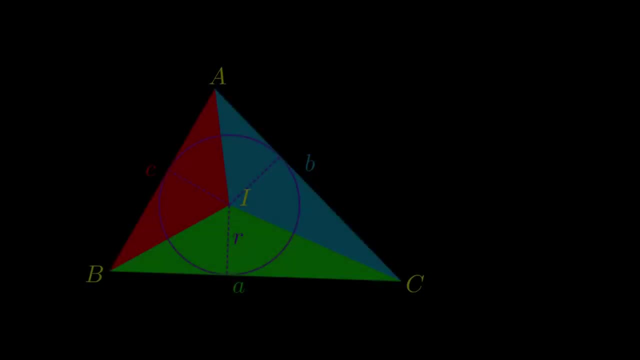 These two proofs rely very heavily on algebra. so are there any other ways to prove Heron's formula without these heavy machinery? These two methods presented below would be more heavily reliant on geometry. instead, These two proofs, both in turn, rely on these two results. 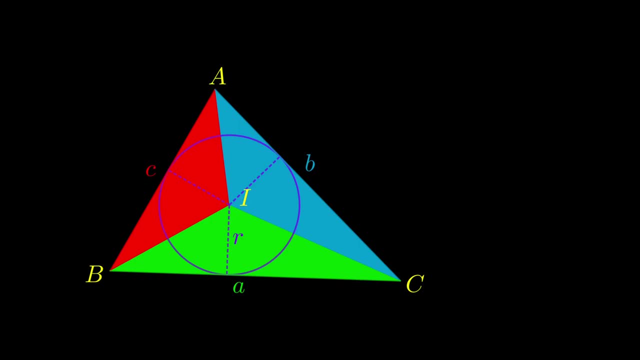 First, we have a novel way to calculate the area of a triangle using this diagram, where i here is the in-centre of the large triangle. To save space, we use the notation that s, with the subscript xyz, meaning the area of the triangle stated. Then we have the large. 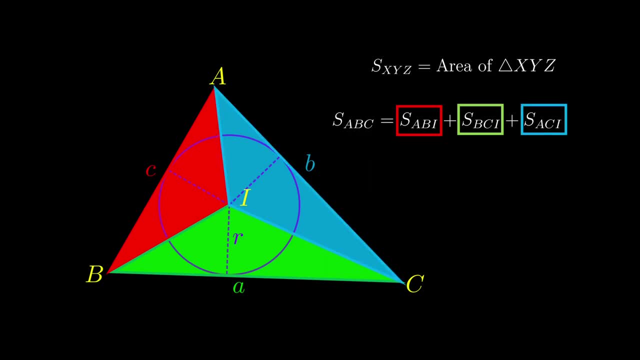 triangle being the three smaller triangles combined, And we can apply half base times height to each of the smaller triangles. This is the same method used in the previous example, And get the area can also be calculated by the product of r, the in radius. 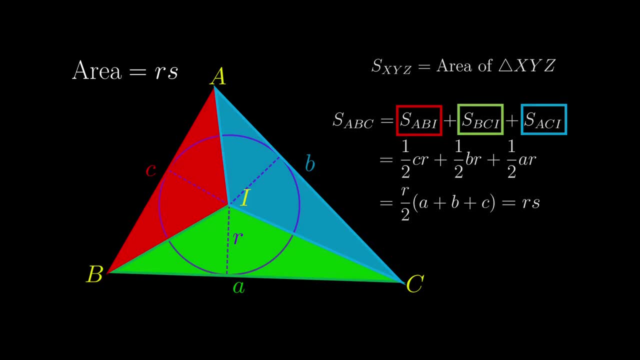 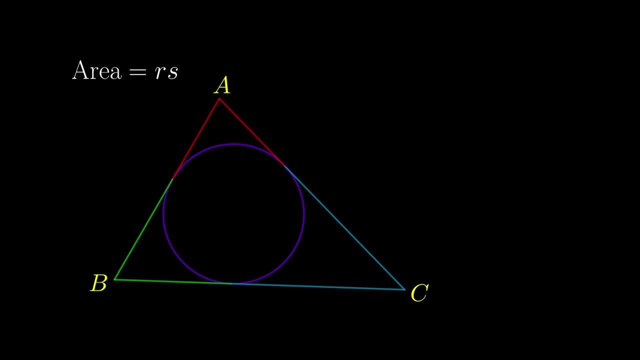 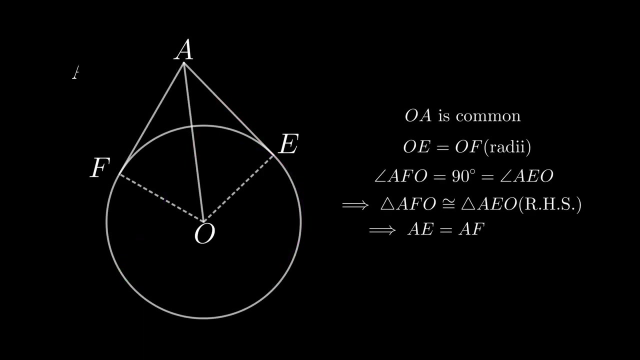 and s the semi-perimeter. Another result we need is a geometric meaning of s-a, s-b and s-c. In this diagram, line segments with the same colour are of the same length. If you really want, here is a simple justification. Pause the video if you want. Form the diagram. you can see that these triangles are in same colour with the same length. First, the color of the triangle should be a horizontal line as the color of the triangle. Then the line segments should be a gradient line, regular line lines. No line segments, so no geometric direction, No vertical line lines, and that's it. And this mean the diagram should be in a particular form. From the diagram we can see that these two shapes are not. vemos the objects as they stand. 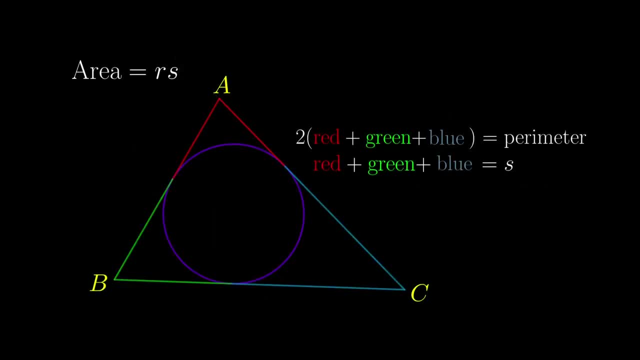 From the diagram it is now easy to see that on the perimeter red, green and blue segments have appeared twice, so they add up to the perimeter and then divided by 2.. Now, if we concentrate on side AB, we have red and green segments adding up to C and 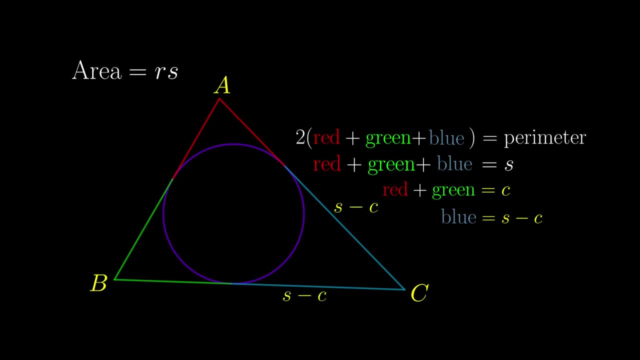 so the blue segment has the length s minus c. Similarly the red segment has length s minus a, while the green one has length s minus b. A good mnemonic is that the segments from A would have length s minus a, from B would. 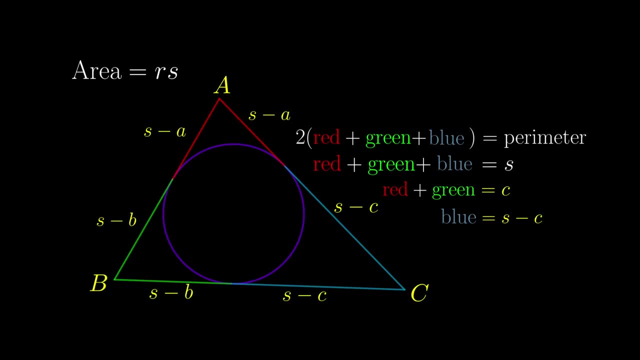 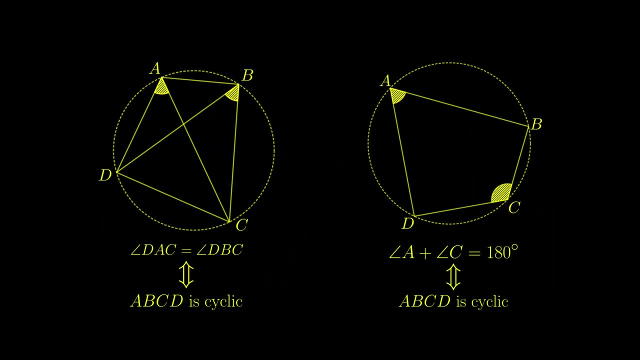 have length s minus b and from C would have length s minus c. Before we start with Heron's original proof, here is just two more results specific to this third proof, where the proof of these results will be at the last part of the video. 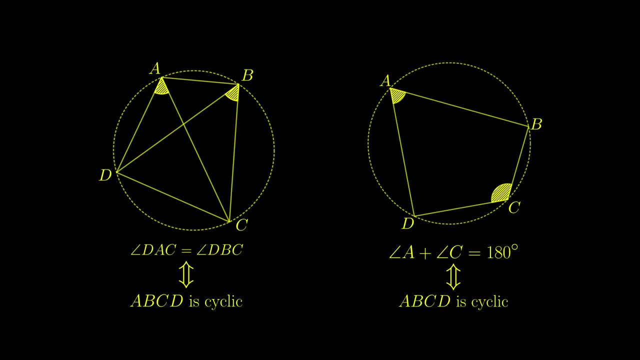 If any quadrilateral fulfills either of the criteria, it can be inscribed in a circle that is cyclic. Conversely, if any quadrilateral is cyclic, it must have these two properties. We name these two results, a and b respectively, for future reference. 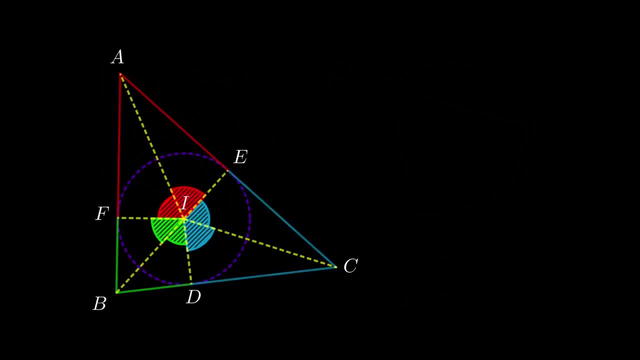 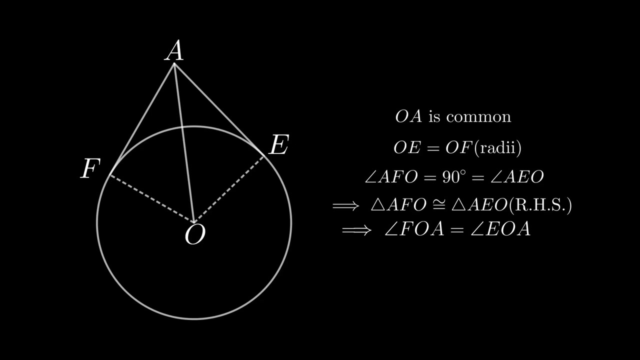 Now we are ready for the proof. First off, we have this colourful diagram where the angles of the two quadrilateral segments are the same at the centre are of the same size if they are coloured the same, which can also be easily justified using congruent triangles shown previously. 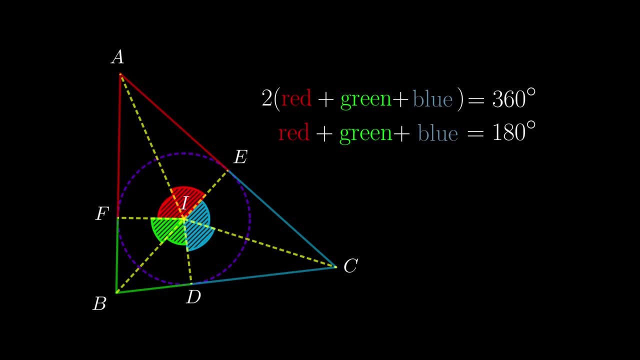 So now, considering the angles around the point I, we have two angles of each colour, and so red, green and blue angles add up to 180 degrees. We now associate the red angle to be the angle AIE and the combined green and blue angles to be angle BIC. Then we can: 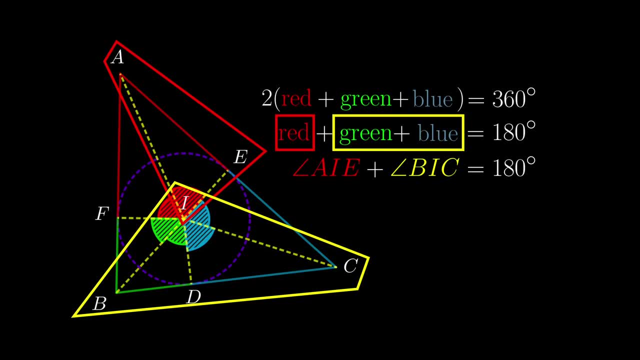 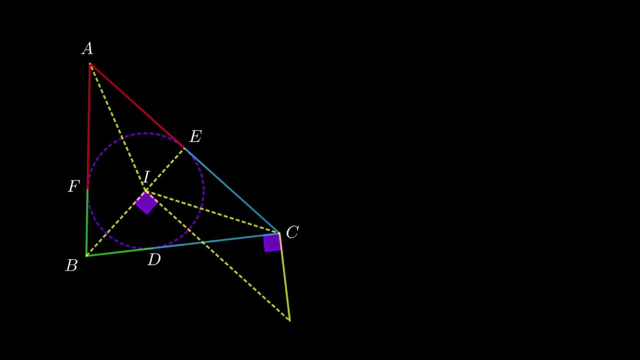 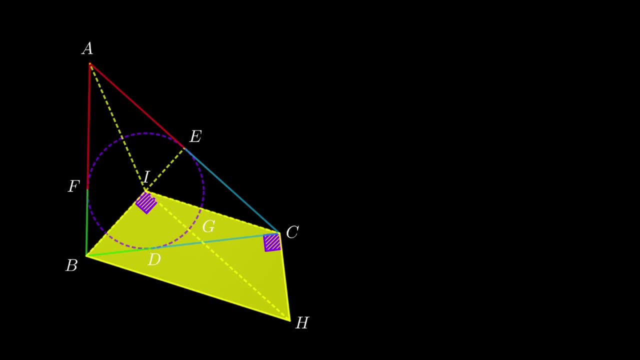 And this appears to be an obvious declension- that will luxury rook or even even to the above. The percentage which deeds wants to determine the threshold of inch through ICH B for ICH would be cyclic, because the two purple angles are the same and we have property A. 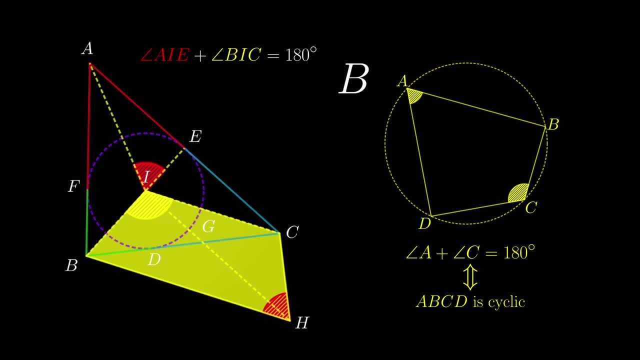 Now, since it is cyclic, These two opposite angles would add up to 180 degrees due to property B, The progressed angle is the amount and, from what we have discussed, the two angle, which does not correspond to indexing group. its now is our ideal bet. 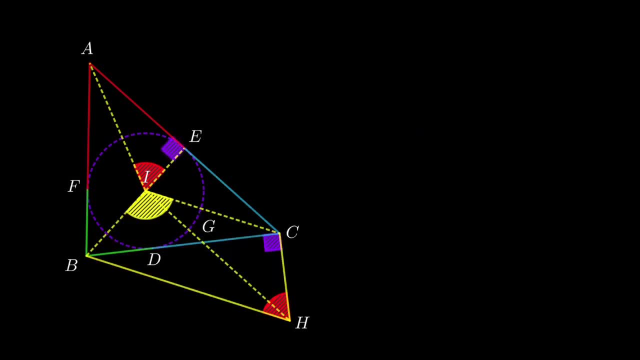 The covered one over is the野r stepp. From what we have discussed, the yellow and red angles in the middle add up to 180 degrees- two right angles. we can conclude that these two grey triangles are similar. There are just two more pairs of similar triangles which are easy to identify. 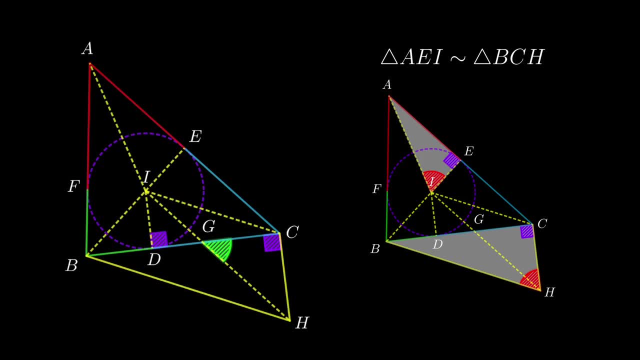 Firstly, in addition to the right angles, we also have these two vertically opposite angles, So it is enough to prove the similarity. These two are also similar because the yellow and red angles add up to angle BIG, which is, by construction, 90 degrees, And similarly, in a triangle, the yellow and red 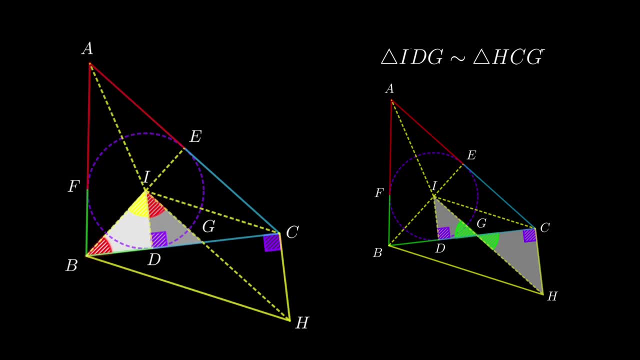 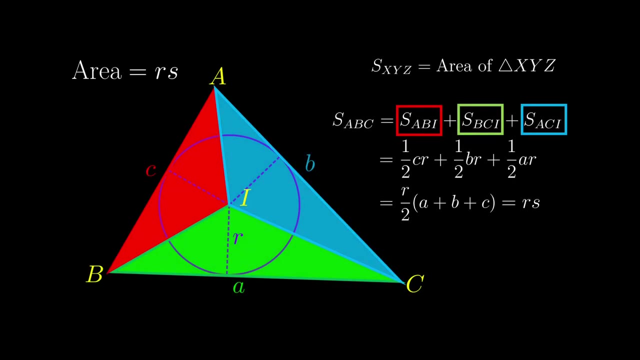 angles also add up to 90 degrees, so the two red angles are of the same size. With the right angle, we can also prove the similarity of these two triangles. It might be a lot to take in, so let me summarise what just happened. 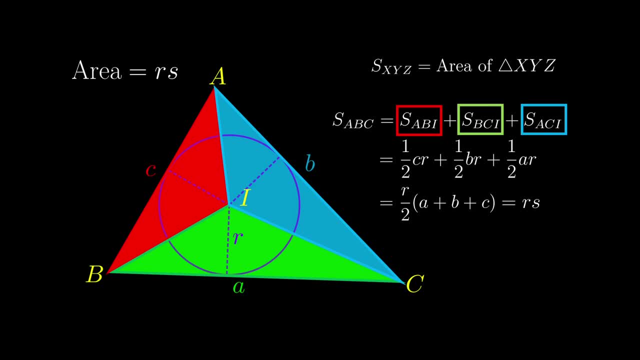 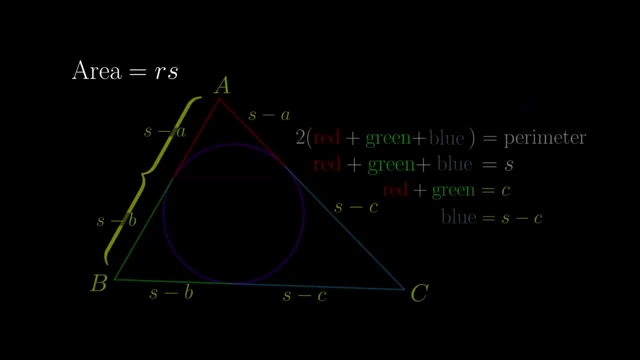 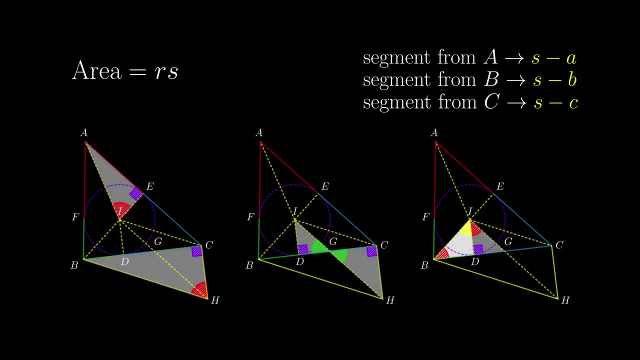 We managed to arrive at the conclusion that the area is the product of R and S, as well as the side lengths expressed in terms of S, A, B and C. Then we proved three pairs of similar triangles. If you don't understand how we came up with these, 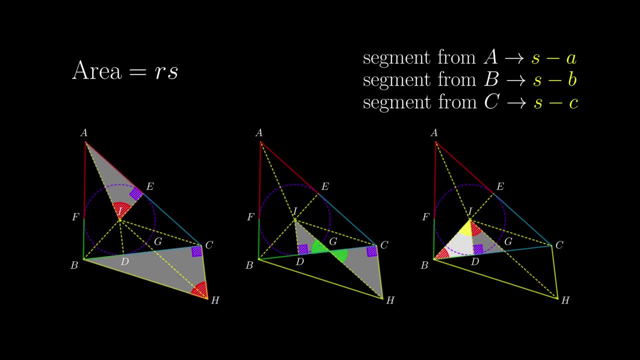 first, don't try this at home. Think over it by yourself, because I assure you that you will gain a much deeper understanding by thinking through this. However, if you have absolutely no idea, then of course you should replay what we have done and pause where necessary. We now move on. 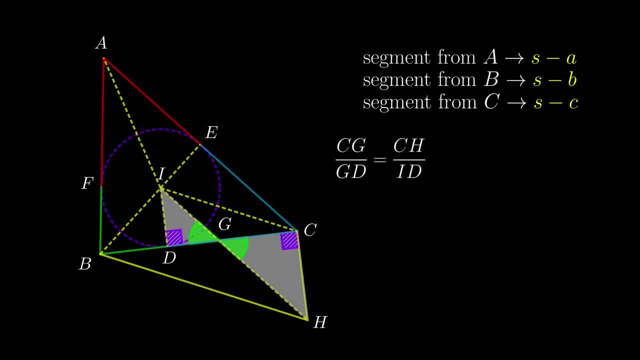 From this pair of similar triangles. we have this proportionality of sides. Now, since both I-D and I-E are the radius of the circle, they are of the same length, so we can replace I-D by I-E. Now we look at another pair of similar triangles. 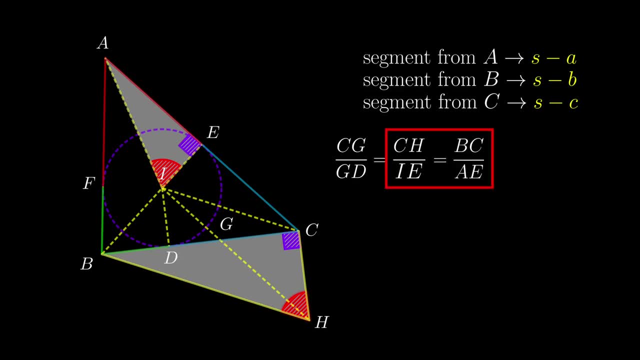 We have another proportion of sides. We can now replace B-C by the symbol A and from the results we obtained, we have A-E to be S-A. Now we add 1 to both sides and we write 1 in different forms. 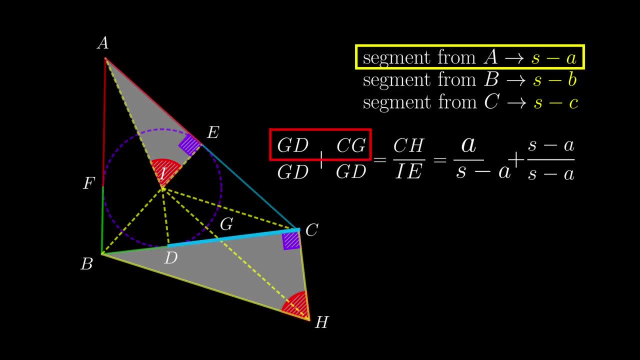 Now the sum of G-D and C-G is from the diagram C-D and from the results previously obtained, it is actually S-B. Now focus on the right side, which is S over S-A. Rearranging: we have this formula. We are quite. 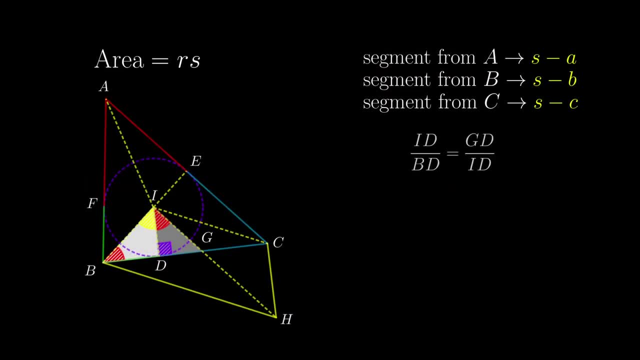 close. now From this pair of similar triangles we have this proportion of sides. Since I-D is the in-radius, We replace I-D by R and from the previous results we have B-D to be S-B. Rearranging we get this formula Combining with the result derived a minute ago. we first multiply. 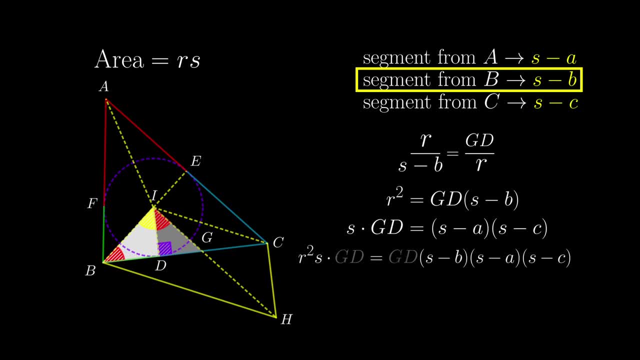 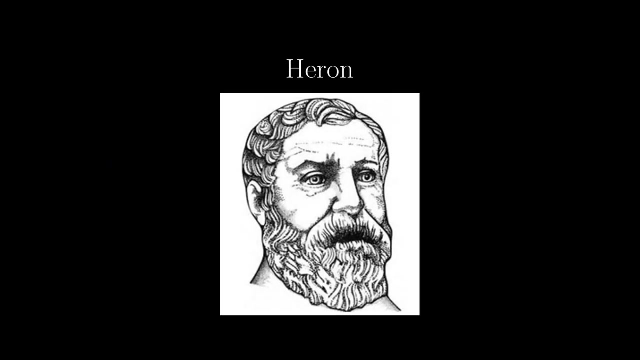 both models. Cancel G-D on both sides, then multiply both sides by S, Then square-root both sides. Churchill's Law R times S. we finally have the Heron's formula. Now, given how complicated this proof is, we really need to give a round of applause to Heron to come up with the entire proof. But 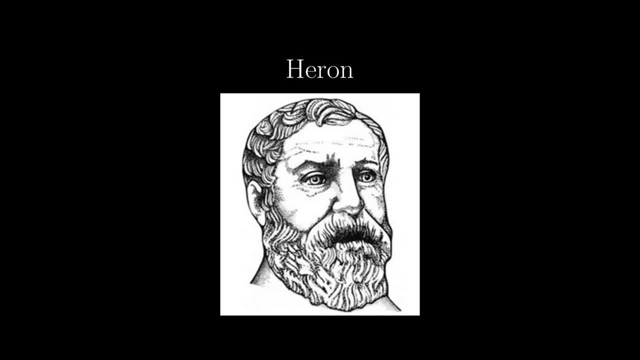 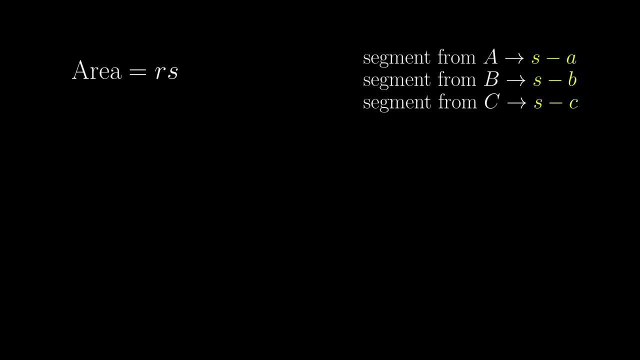 now we have much less complicated geometric proof. after so many years, We would still use these two results. First, we construct external angle bisectors of B and C which will intersect at the point which we call IA, Since angle bisectors are the 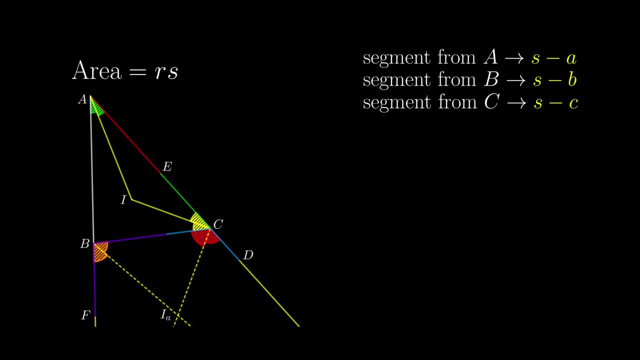 collections of points that are equidistant from the two lines that create the angle, which can be proved pretty easily. that means IA is equidistant from BF, BC and CD and so on, So also lie on the angle bisector of A And of course, because of the equidistance we 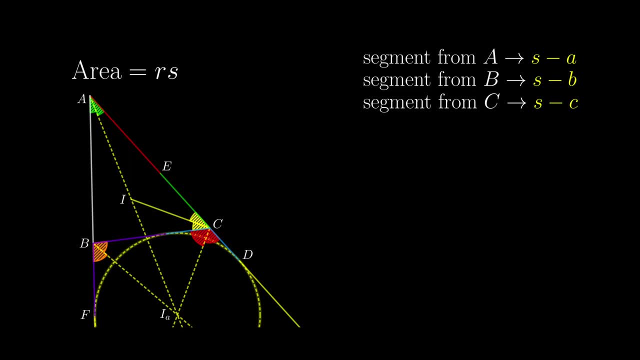 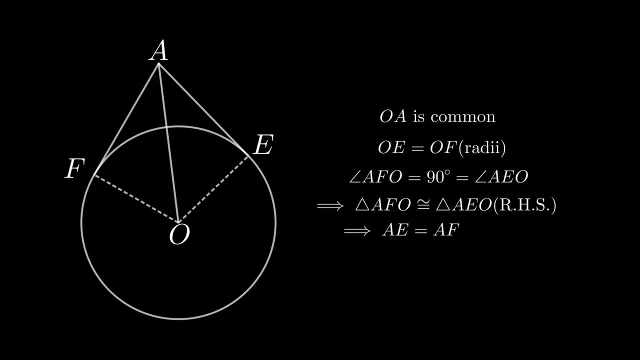 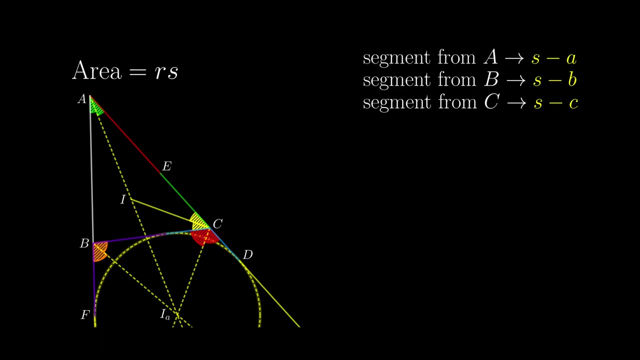 can draw a circle, just touching the sides, Since we have previously demonstrated that the tendential segments from a point are of the same length. we have the pairs of blue and purple segments having the same length And so they add up to length BC At the same. 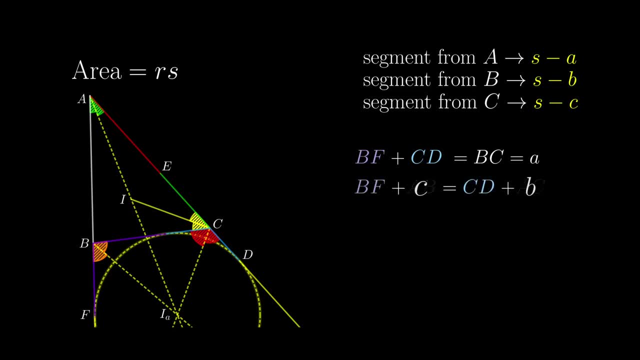 time we have A and B. In order to polite them, I tried to put A F equal to A D, And so we have this relation Rearranging. we get the difference between these two cheap links. By subtracting the second relation from the first, we have this. What's interesting is that we of course have 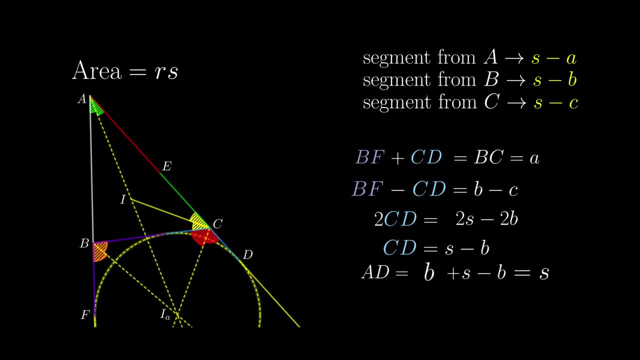 AD as the sum of these two links, which can be found to be S. so we give S its geometric meaning unconditionally: Iました. Now we have this pair of triangles to be similar, which is pretty evident from this, from the green common angle and the right angles. So we have this proportion of sides. 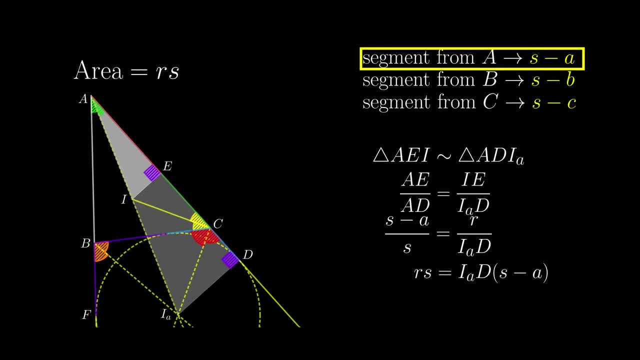 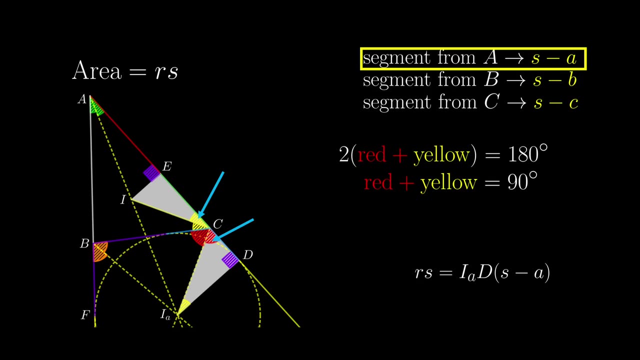 Since we have the previous result, we turn AE to S-A and then we have this formula For this pair of triangles. we observe that around vertex C, red and yellow angles appear twice, adding up to 180 degrees. so these two angles add up to 90 degrees At the same time. 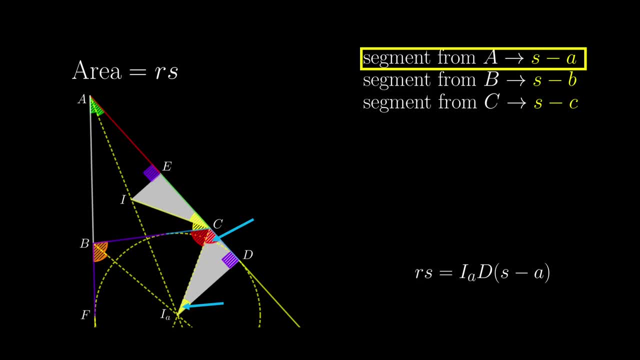 these two angles add up to 90 degrees because of how angles sum up in the triangle. Combining with the two right angles, we can prove the similarity of the two triangles. Now we write down the proportionality of the sides and use the results we have before and we have this relation.